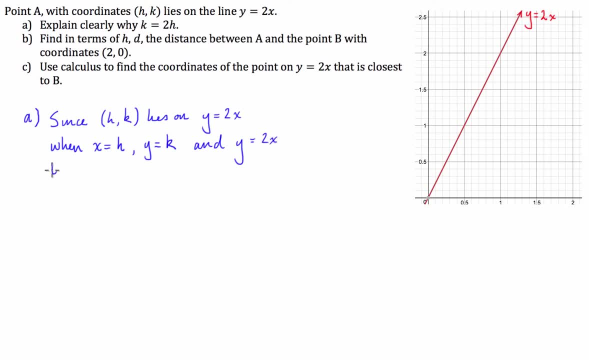 2x. you just can write then comma y is k must be equal to 2h, Full stop, And that's all you'd have to write. But it's important that you say that, since you've got a point that lies on this line and we can substitute the values for x to h and y to k. 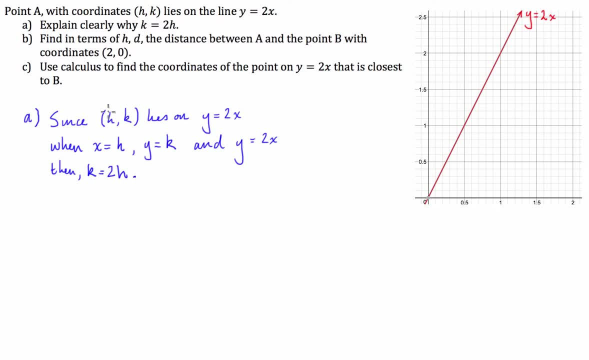 we can then substitute k into 2h. So basically we're saying, because this lies on this, we can substitute the h's for the x's and the k's for the y's. So not too complicated. but, as I said before, the way you word your answer is crucial in this case. 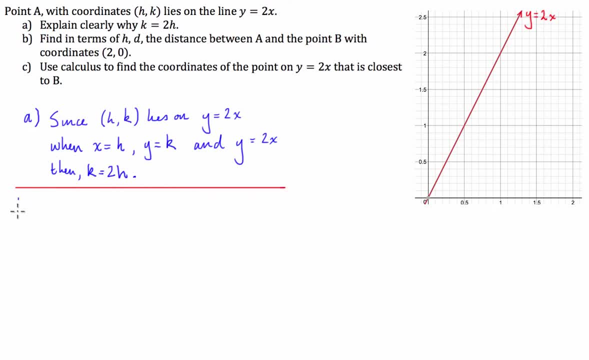 So what is the next part of the question asking us to do? Find in terms of h, d, what is the distance between a and the point b with coordinates 2 comma 0?? Okay, so I'm guessing. that's why we've got this graph here. So 2 comma 0 is here. 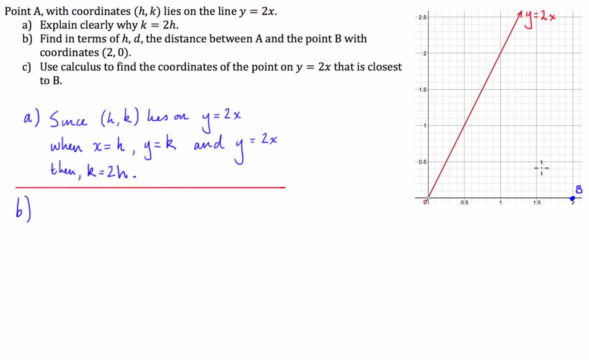 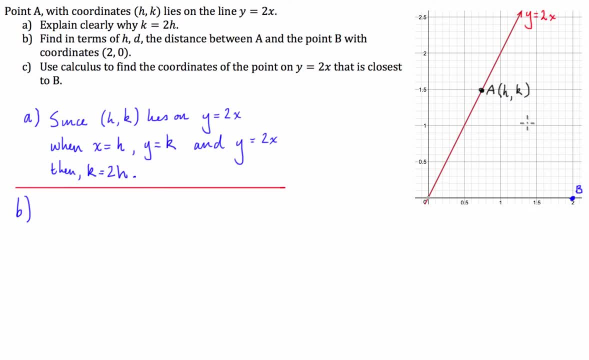 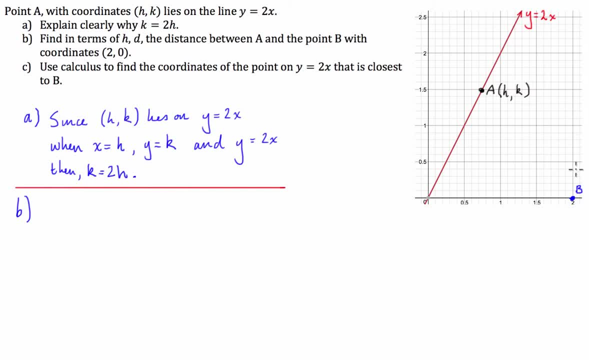 these two points in terms of h. So thinking back, guys, to your sort of junior high school days, you will hopefully be aware of this distance formula, which looks like a lot like a- you know- Pythagorean identity, where we have the distance between two points. 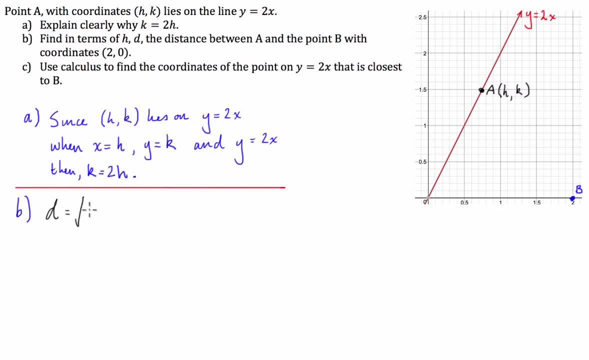 and the distance between two points is equal to the square root of the x-coordinate of one of the points minus the x-coordinate of the other point, all squared, plus the y-coordinate of one of the points minus the y-coordinate of the other one of the points squared. 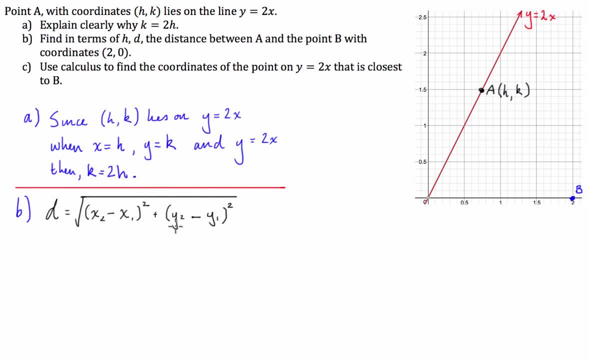 So what we can do now is we can substitute in the values that we know, So we can say that d is equal to the square root of x2.. Let's call that this one here. This is going to be our number two, and this one here is going to be our number one. 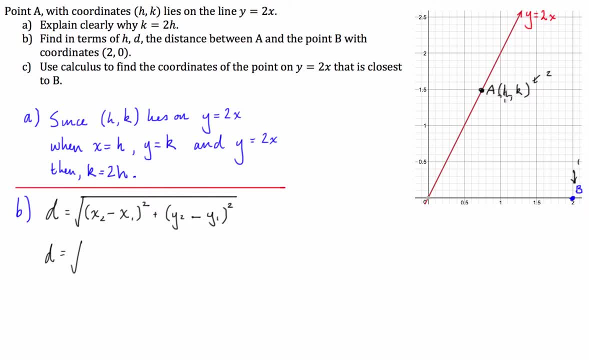 So x2 is going to be equal to h. So I'm going to say: this is equal to the square root of h. take x2.. x1, which is just 2, all squared, plus y2, which is k, or I could write 2h, because that's what we. 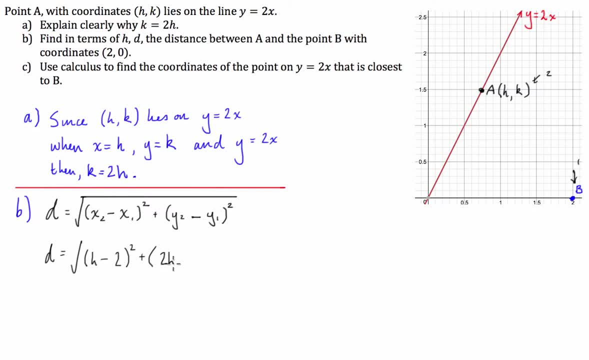 determined up here. subtract zero: squared: Cool, So we can simplify this a little bit. So we have the square root: h take 2, all squared. Hopefully, you guys are well aware that well, I have a lot of students that still manage to mark this up. h take 2, all squared is equivalent to: 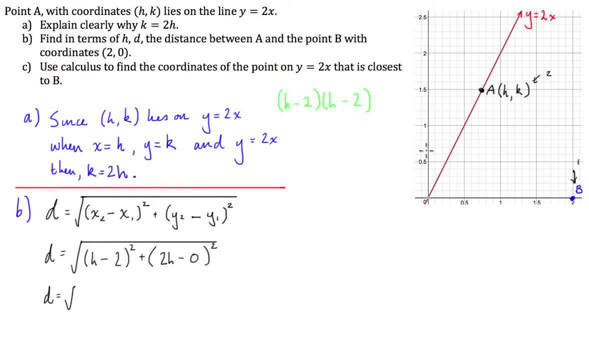 this, And so if you do our first inside-outside last here, you're going to get h squared, take 4h plus 4.. So we can put that under the bracket here. We can say: this is h squared, take 4h plus 4, and then 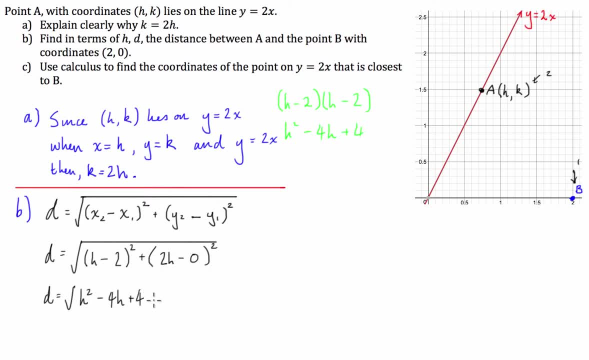 here we've got 2h all squared, because the zero makes no difference. So this is just going to be: 2h squared is 4h squared, And then I put all of that under a square root sign And finally, 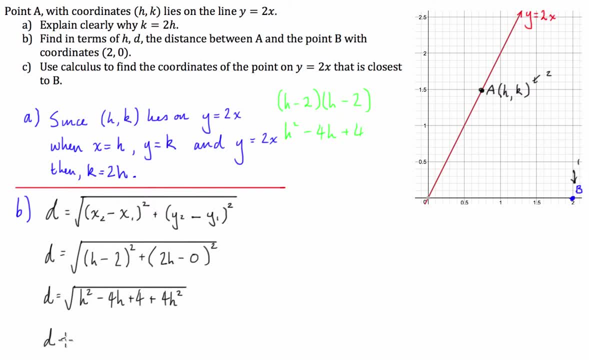 combine our like terms, We have: d is equal to the square root, h squared plus 4h. squared, is you guessed it? 5h squared minus 4h plus 4, all square rooted. Cool, So that's. we've found, in terms of h, the distance between this point b and this point a. 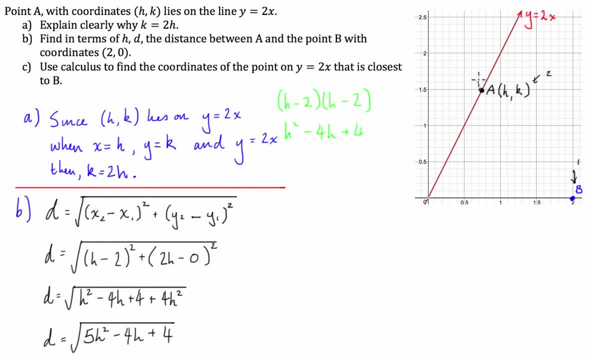 here which can move along this line. So a could go, you know, up in this direction, or it could go down in this direction. Okay, so c, let's just separate these out a little bit. So we have part c. use calculus to find the coordinate of the point on. y equals 2x. 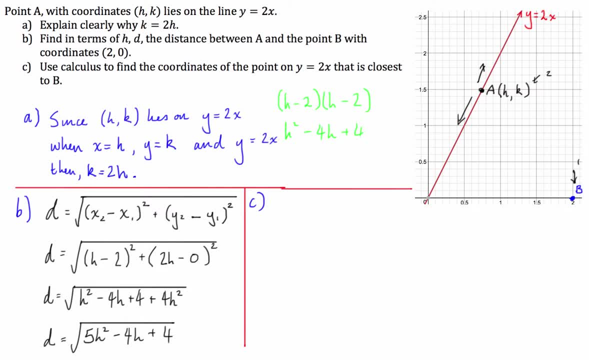 that is closest to b. Okay, so what is that? What is the goal in part C? Well, we have to find the point in terms of H that minimizes D or this value here. So let's get cracking To do this using calculus. they kind of give it away. 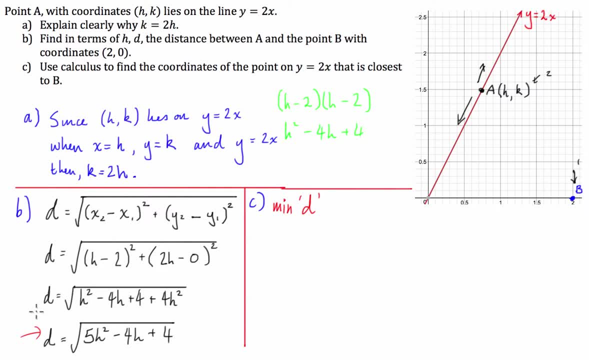 What we need to do is we need to find the derivative of D, So we need to find D dash with respect to H. Now, hopefully you guys are aware that, rather than putting a square root sign, the equivalent to this is: I can write, put this in brackets and go 5H squared. 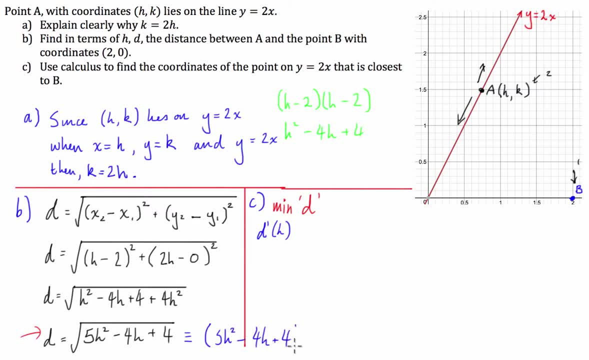 take 4H plus 4, all to the power of 1 half. So these two representations are equivalent. So this is easier for me to picture the derivative for. So I hope you don't mind me going with this one. 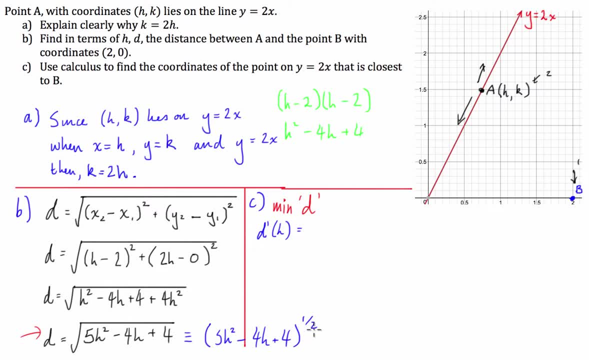 So the derivative of this. we're going to use the chain rule. We take the half down the front so we have 1 half. We leave the inside constant, 5H squared. take 4H plus 4.. We lower the power by 1, so it's going to be negative, 1 over 2.. 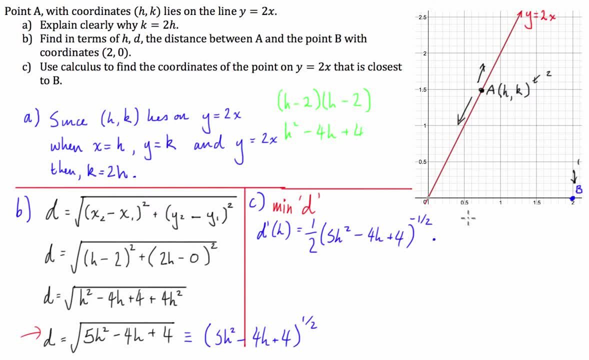 Then we multiply it by the derivative of the inside function, which is 1 over 2.. So we're going to use 10H minus 4. And we'll put that in a bracket to make it easier to separate Cool. 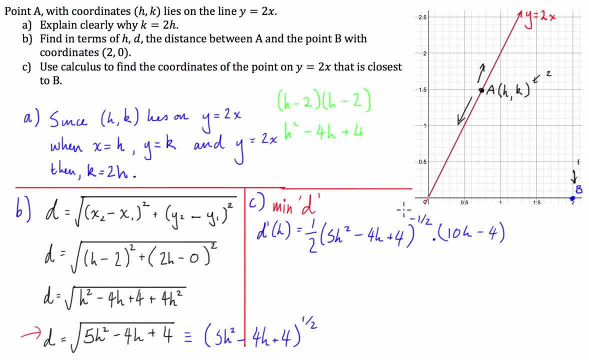 Now we have to simplify this, ie like get it into a usable form, Because that's a negative half power. it's going to go in the denominator with the 2. And I'm going to be left with 10H minus 4,. 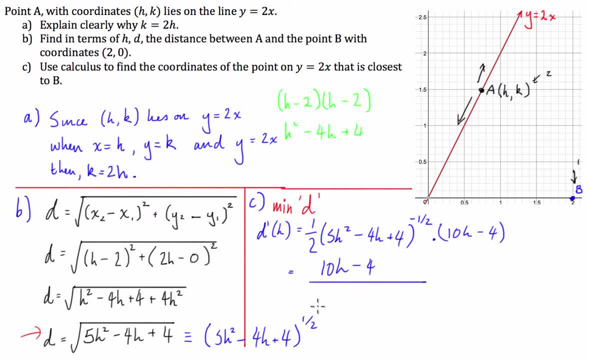 divided by 2 times the square root of 5H squared minus 4H plus 4.. Okay Now I hope you guys are aware that to find the derivative, or why we find the derivative, is to minimize D, That's when this derivative equals 0.. 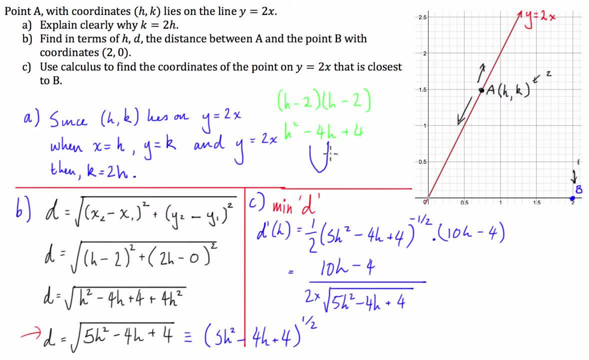 So it's when we have a turning point in our function. ie there. So what we do is we're going to make this equal to 0. And hopefully you guys have some understanding of rational functions and how they work. 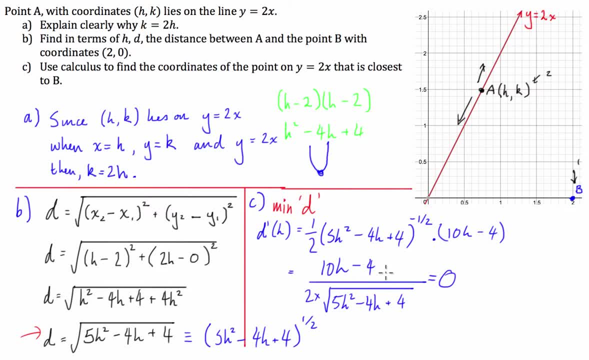 So the only way this is going to be equal to 0, is when the numerator is equal to 0. If the denominator equals 0, then the function doesn't make sense. So what we can do to simplify our algebra journey is we're going to say: well, this: 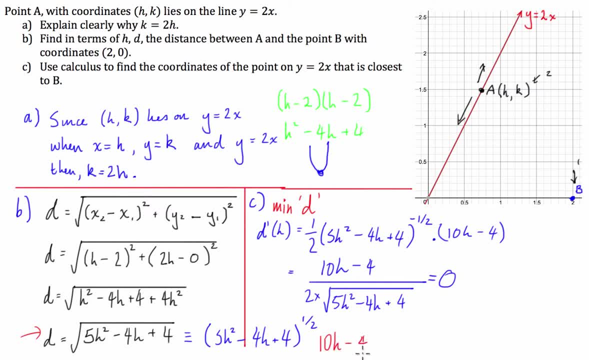 can be simplified down to 0.. So we're going to say: well, this can be simplified down to 10H. take 4, has to equal 0.. So what I'm going to do is I take 4, across to the other side and I divide it by 10,. 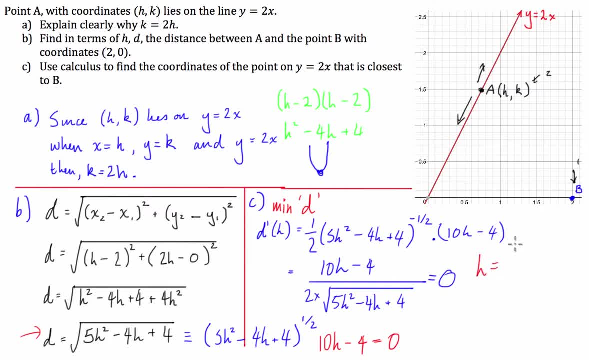 and I get: H is equal to 4 on 10, which is equal to 0.4.. Great. So that's my H value. I can also find my D k value, because I know that k is equal to 2h, so I can say, therefore, k is equal. 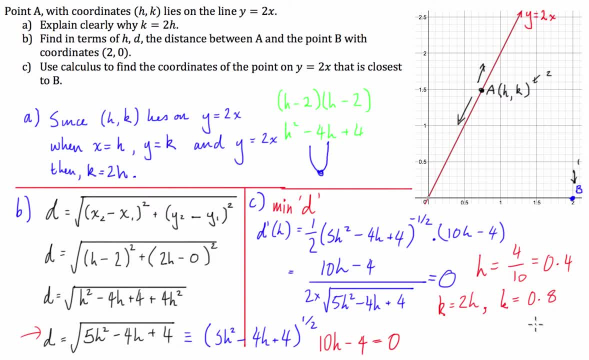 to 0.8 and finally, to ensure that this is a local minimum, I'm going to draw just a small gradient table, I think would be the best term for it, so I'm just going to go cool. so what I have at the top is I have h, and then I've got d dash of h and I 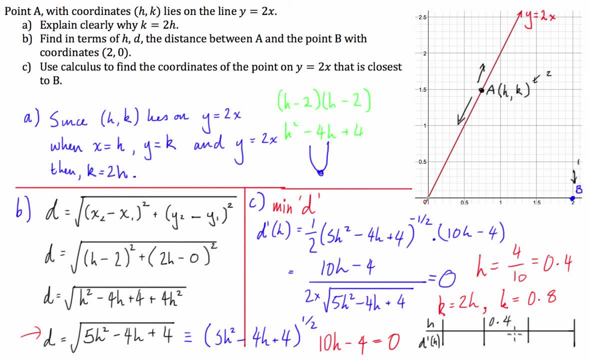 know when h is equal to 0.4. and then I've got d dash of h and I know when h is equal to 0.4. the derivative is 0 when h is equal to anything less than 0.4, so 0.4 coming in. 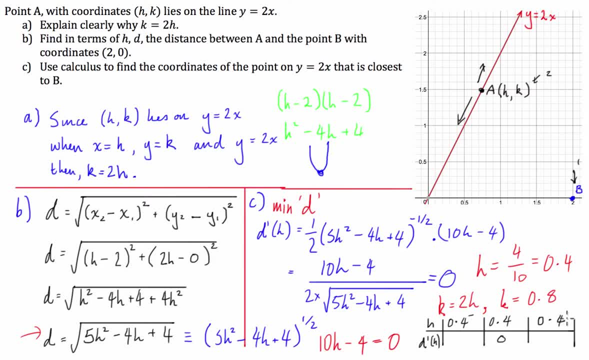 from the negative and 0 and anything greater than 0.4. we have to figure out what these are going to be. so, with this table, what we're going to do is we're going to go. well, if h is anything less than 0.4, let's say 0.2. so I substitute: 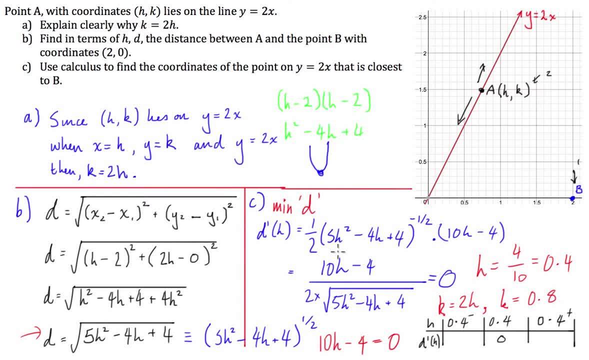 that into my little function here. this is the numerator is. the only thing that really matters here is I go: well, if 10 times 0.2 is 2 minus 4 is a negative number, so the derivative is going to be negative. let's say, a number that's greater than 0.4, 0.5, 0.5 times. 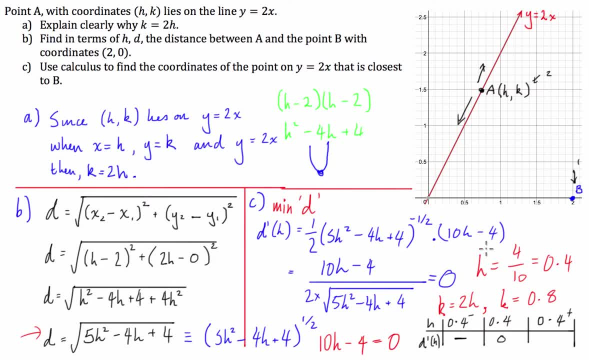 10 is 5, take 4 is 1, so that's positive. so what that means is that our graph is negatively sloped. it then goes to 0 and then it is positively sloped, a minimum. so, guys, what we can say for the answer for C- I've sort of run out of space here- is to find the 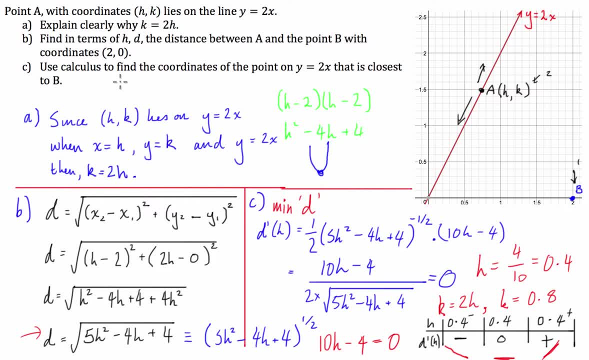 coordinates, the point y equals 2x, that is closest to B. I'm going to say that this is equal to. so a has the coordinates 0.4 or 4.4. so that's the equation. here this equation is going to be 0.4 divided by 7, so we don't use the 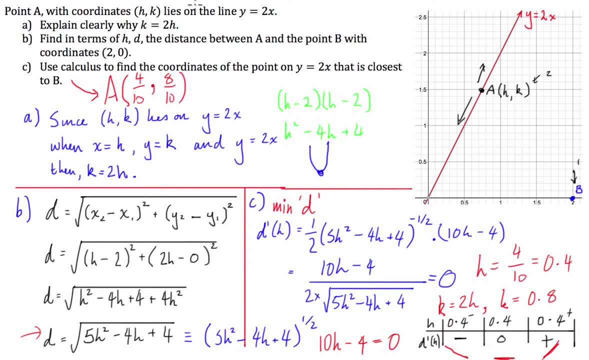 Y and the y is going to be 0.5. it is going to be a negative, the pre-completion equation is going to be 0.5 and the mean times 0.5 is going to be 0.5, so we can. 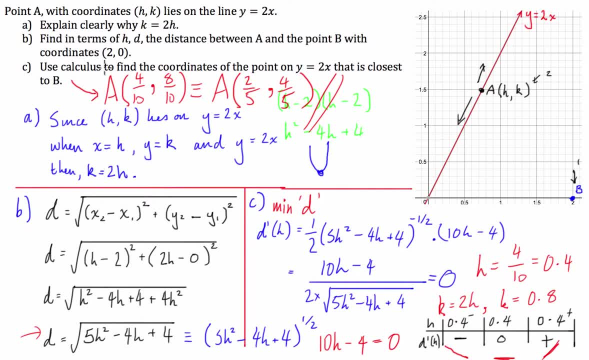 just simply do the same thing here: 0.4 is 20 times 0.5, and then 4 times 0.5 is going to be 0.5. so that gives us what we're going to call the Variable 4 on 10. 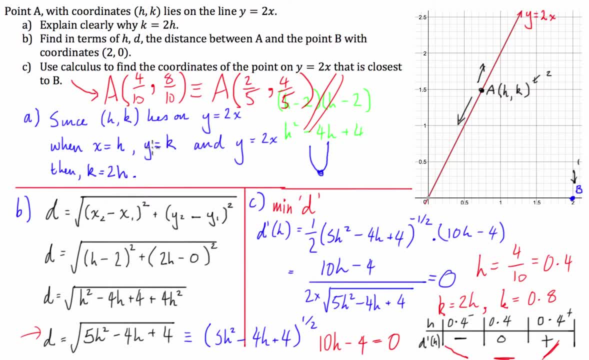 different. A is more of a sort of an understanding of basic principles, basic concepts and making sure that you can explain yourself logically. So you've got to set up a logical argument here with what the premise is, what you're then proposing and then what its implications are.